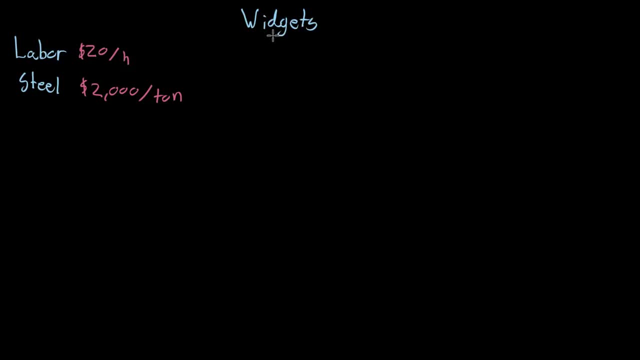 And then you've had your analysts work a little bit on trying to model the revenues you can make with your widgets as a function of hours of labor and tons of steel. Now let's say the revenue model that they've come up with: the revenue as a function of, you know, hours of labor. 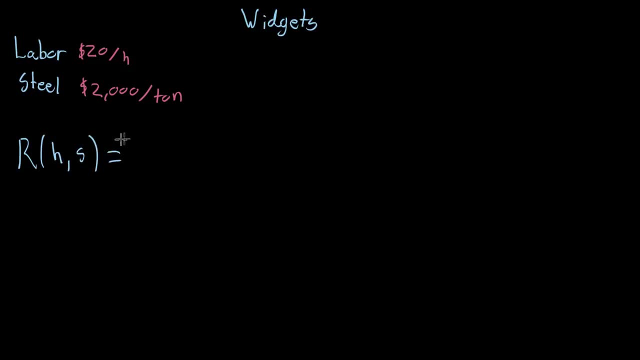 and then S for steel, let's say, is equal to about, you know, 100 times the hours of labor to the power 2- 3rds, multiplied by the tons of steel to the power 1- 3rd, If you put in a given amount of labor. 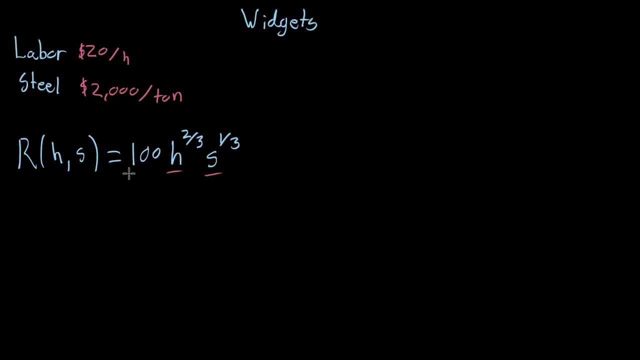 and a given amount of steel. this is about how much money you're gonna expect to earn, And of course you wanna earn as much as you can. but let's say you actually have a budget for how much you're able to spend on all these things. 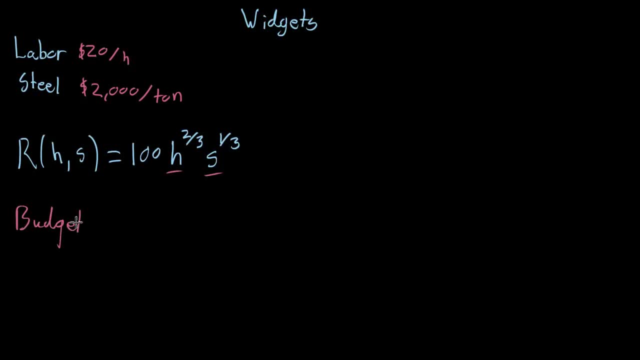 and your budget. the budget is $20,000.. You're willing to spend $20,000 and you wanna make as much money as you can according to this model. based on this, Based on that. Now, this is exactly the kind of problem. 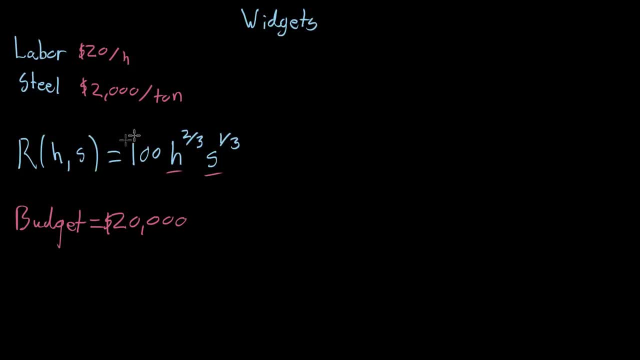 that the Lagrange multiplier technique is made for. We're trying to maximize some kind of function and we have a constraint Now. right now the constraint isn't written as a formula, but we can pretty easily write it as a formula, because what makes up our budget? 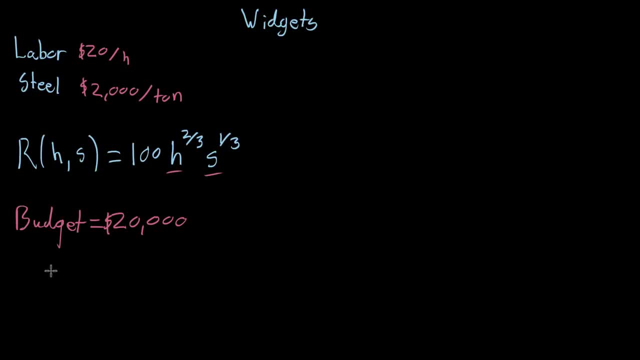 Well, it's gonna be the number of hours of labor multiplied by 20, so that's gonna be $20 per hour multiplied by the number of hours you put in, plus $2,000 dollars per tons of steel. times the tons of steel that you put in. 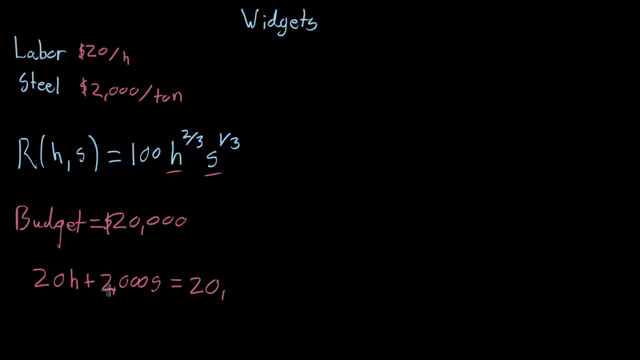 So the constraint is basically that you have to have these values equal $20,000.. I mean, you could say less than right, You could say you're not willing to go any more than that, but intuitively and in reality, it's gonna be the case that 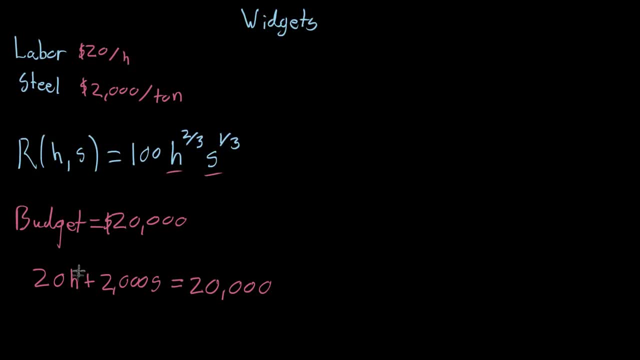 in order to maximize your revenues, you should squeeze every dollar that you have available and actually hit this constraint. So this, right here, is the constraint of our problem, and let's go ahead and give this guy a name, the function that we're dealing with a name. 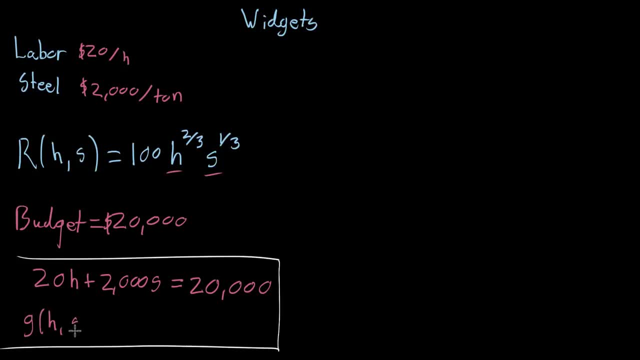 and I'm gonna call it g of hs, which is gonna be that guy. And now, if you'll remember, in the last few videos, the way we visualize something like this is to think about the set of all possible inputs. so in this case you might be thinking about the hs plane. 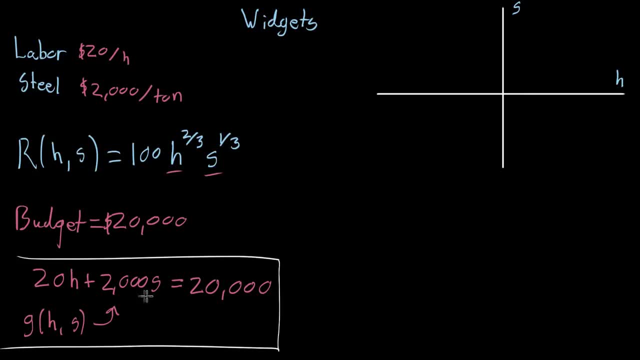 the number of hours of labor on one axis, the number of tons of steel on another. and this constraint? well, in this case it's a linear function. so this constraint is gonna give us some kind of line. It tells us which pairs of s and h 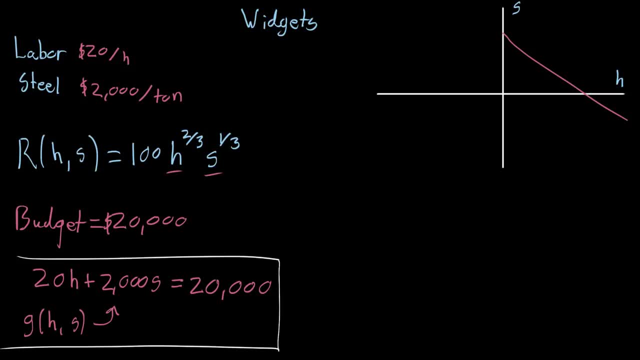 are gonna achieve that constraint And then the revenue function that we're dealing with will have certain contours. you know, maybe revenues of $10,000 have a certain contour that looks like this and revenues of $100,000 have a certain contour that looks like this: 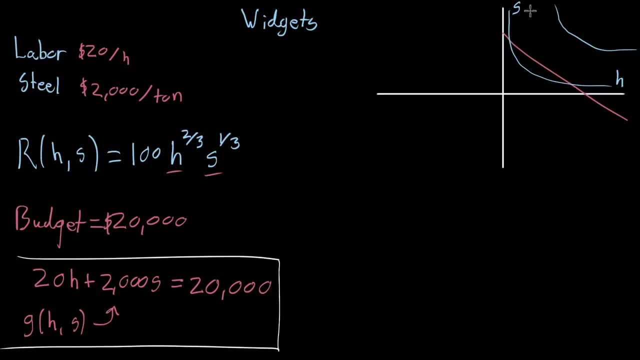 But what we want is to find which value is barely touching the constraint curve, just tangent to it at a given point, because that's gonna be the contour line where, if you up the value by just a little bit, it would no longer intersect with that curve. 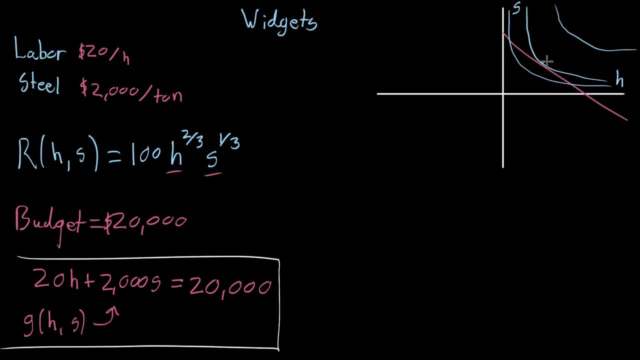 There would no longer be values of h and s that satisfy this constraint. And the way to think about finding that tangency is to consider the vector perpendicular to the tangent line, to the curve at that point, which, fortunately, is represented by: let's see, let me make some room for myself here. 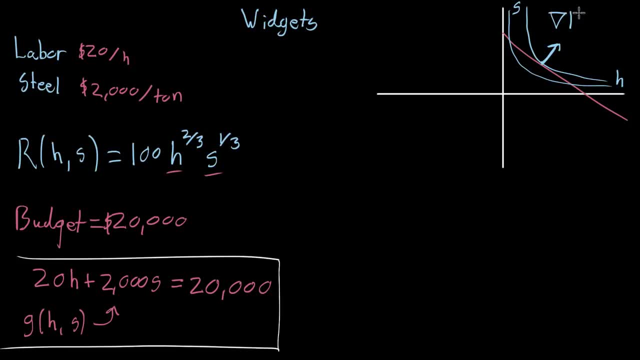 represented by the gradient, the gradient of our r function, the function whose contours- this is the revenue, And what it means for this to be tangent to the constraint line is that there's gonna be another vector, the gradient of g of our constraint function. 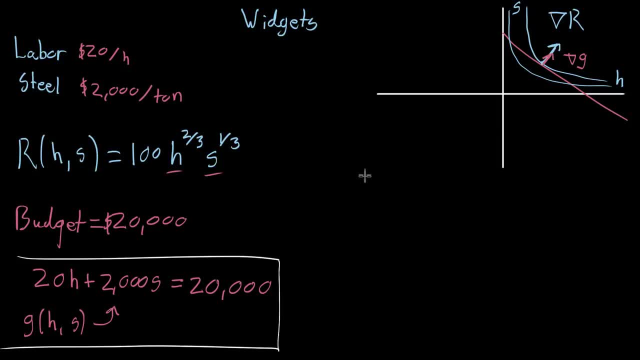 that points in the same direction, that's proportional to that, And typically the way you write this is to say that the gradient of this function is proportional to proportional to the gradient of g, And this proportionality constant is called our Lagrange multiplier. 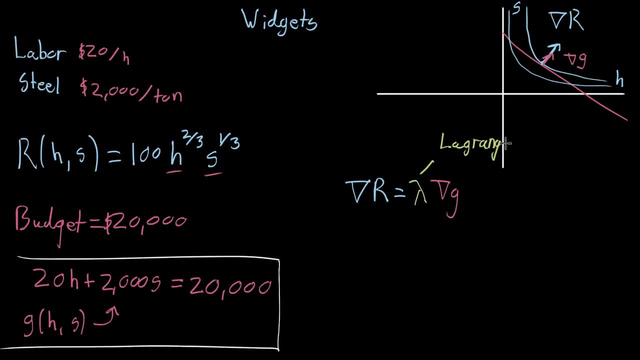 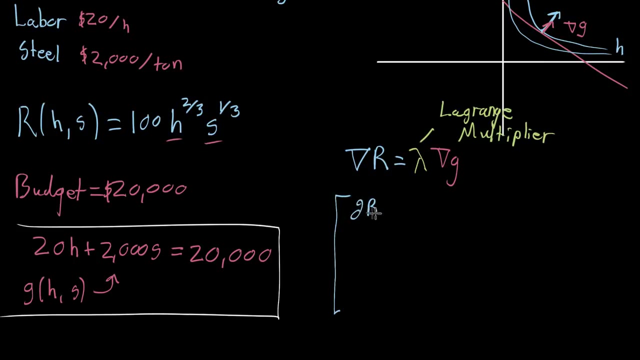 It's called the Lagrange, the Lagrange multiplier. So let's go ahead and start working it out. Let's first compute the gradient of r. So the gradient of r is gonna be the partial derivative of r with respect to its first variable, which is h. 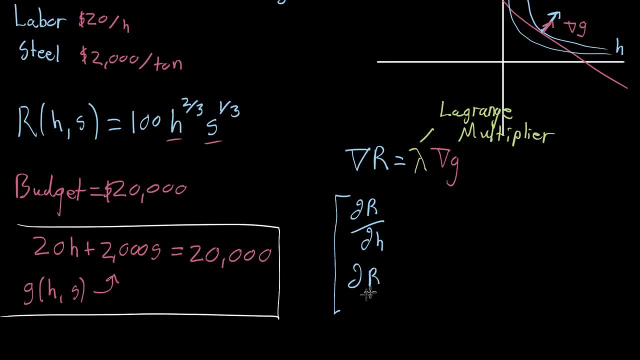 So partial derivative with respect to h, And the second component is its partial derivative with respect to that second variable, s with respect to s. And in this case, that first partial derivative if we treat h as a variable and s as a constant. 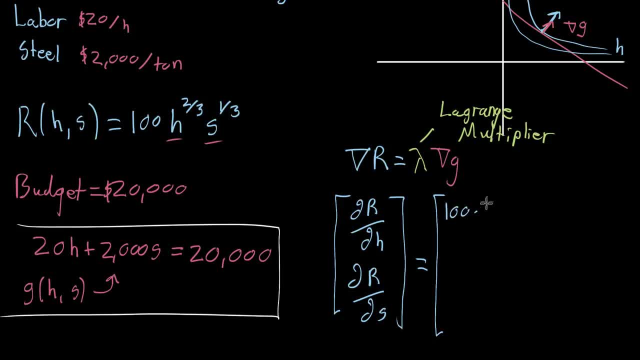 then that 2 3rds gets brought down, So that'll be 100 times 2 3rds times h. h to the power of. well, we've gotta subtract one from 2 3rds when we bring it down. 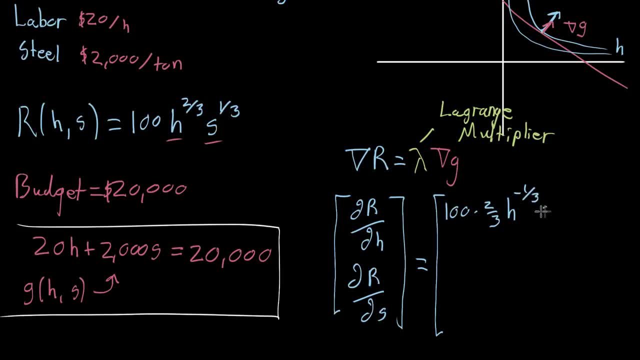 so that'll be negative: 1: 3rd multiplied by s to the 1: 3rd, And then the second component here, the partial derivative with respect to s, is gonna be 100 times. well, now, by treating s as the variable, 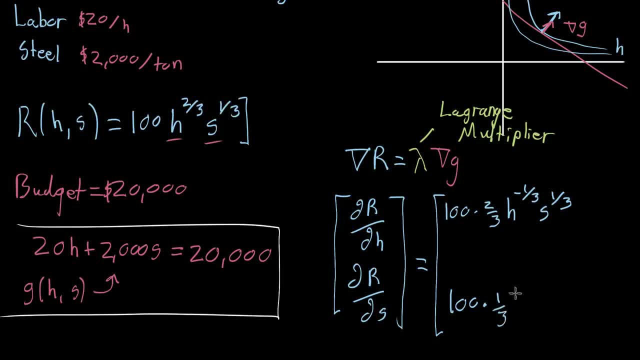 we take down that 1 3rd, so that's 1 3rd h to the 2 3rds. just looks like a constant as far as s is concerned. and then we take s to the 1 3rd minus one. 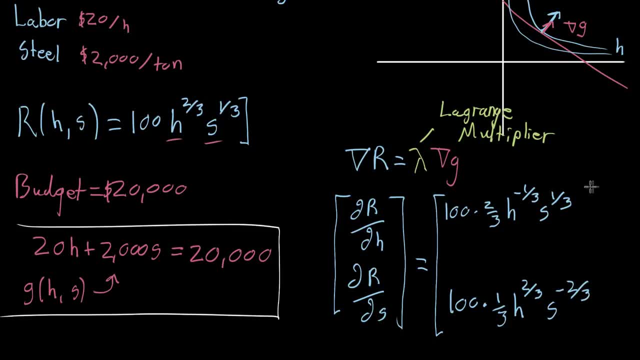 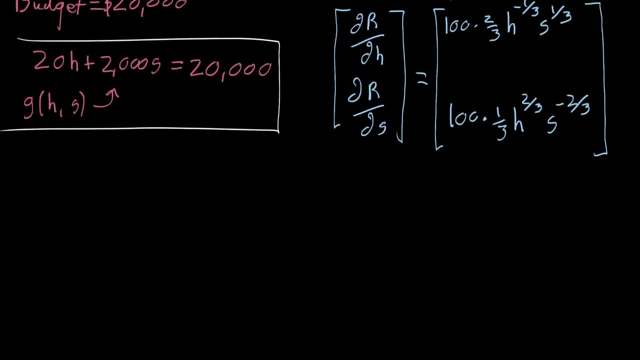 which is negative, 2, 3rds, negative 2, 3rds, Great. so that's the gradient of r, And now we need the gradient of g, and that one's a lot easier, actually, because g is just a linear function. 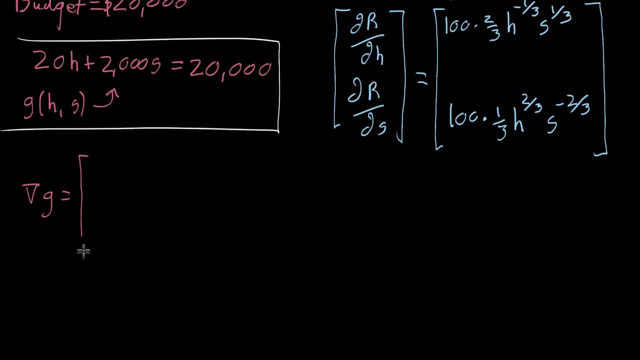 So when we take the gradient of g, which is its partial derivative with respect to h, partial h and its partial derivative with respect to s, partial s. Well, the partial with respect to h is just 20.. The function looks like 20 times h. 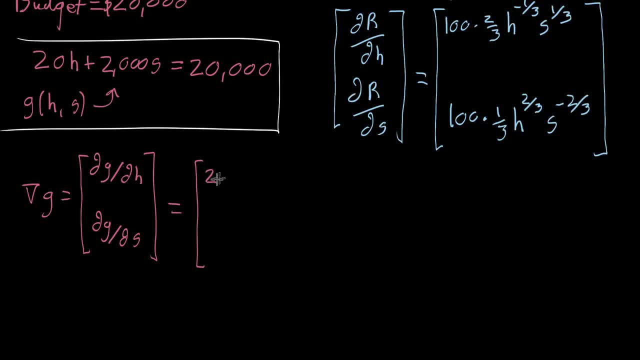 plus something that's a constant, So that ends up being 20.. And then the partial with respect to s. likewise, it's just 2,000, because it's just some constant multiplied by s plus a bunch of other stuff that looks like constants. 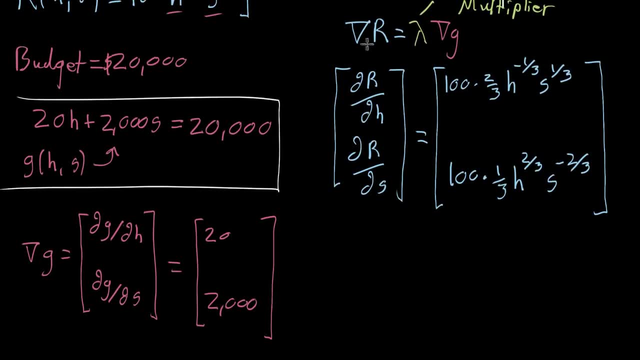 So that's great. And this means, when we set the gradient of r equal to the gradient of g, the pair of equations that we get- and let me just write it all out again- is: we have this top one, which I'll call 200 3rds. 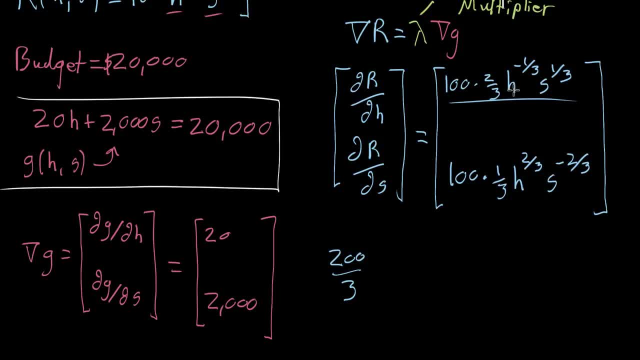 times, and let's go ahead and do a little simplifying while I'm rewriting things here. So h to the 1 3rd is really one over h to the negative 1 3rd. sorry, is one over h to the 1 3rd.